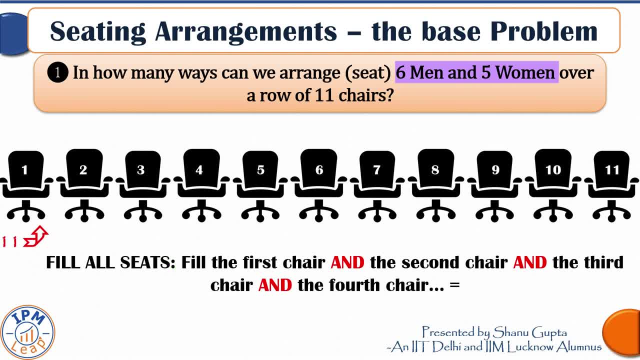 The first chair can be filled in 11 ways. Any one of these 11 persons can get seated here, So 11 ways. Once you fill this chair, there are 10 people left. So next chair can be filled in 10 ways. 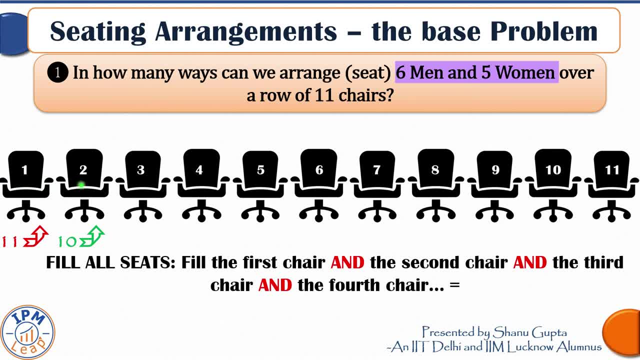 After filling the first two chairs, there will be 9 people left. So third chair can be filled in 9 ways, And so on Fourth chair 8 ways, Fifth chair 7 ways, And we can extend this pattern. 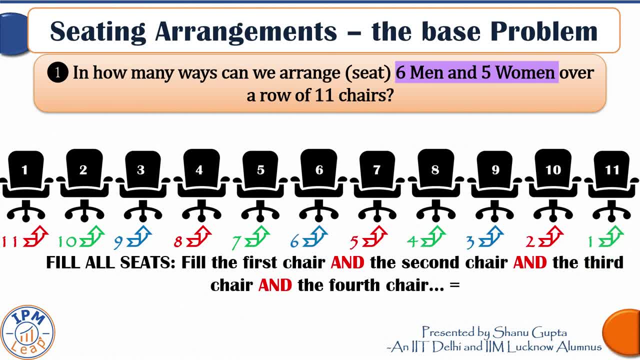 6,, 5,, 4,, 3,, 2.. And finally, for the last chair, there will be only one person left Because everyone else is already seated. So the last chair can be filled in only one way, By using the fundamental rule of counting, since we have to fill the first chair 11 ways. 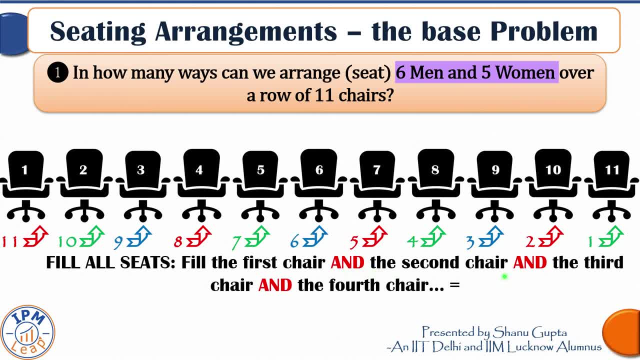 And the second chair 10 ways, And the third chair 9 ways, And so on, And the last chair 1 way, And mace multiply, So together these 11 chairs can be filled in 11 x, 10 x, 9 x, all the way up to 1.. 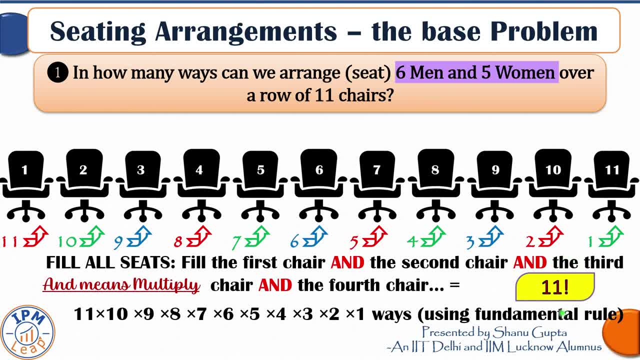 Which means 11 factorial ways. These 11 people can be arranged in 11 factorial ways. It's a huge number. We don't need to calculate it because it's not required in the question And, in general, remember that n different objects can always be arranged in n factorial ways. 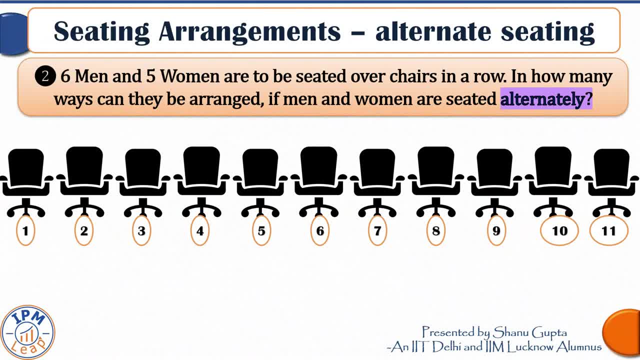 Now let us introduce our first constraint. If we have to seat these 6 men and 5 women alternately, then in how many ways can they be seated? So, friends, this constraint of alternate arrangements makes it clear that we will have to start with a man. 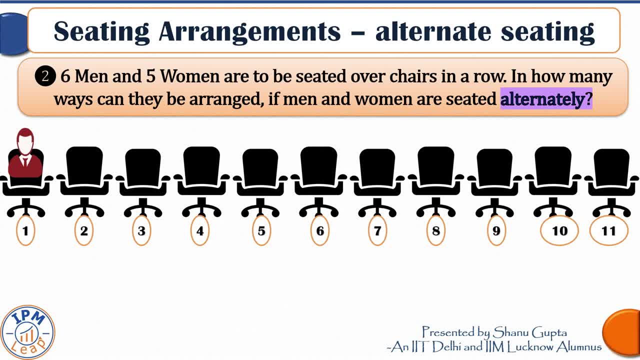 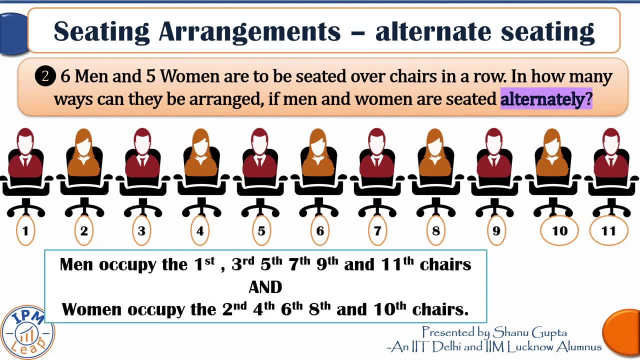 Because if we start with a woman, there will be 2 men left at the end of the row. So alternate arrangements essentially means that men occupy the 1st, 3rd, 5th, 7th, 9th and 11th chairs. 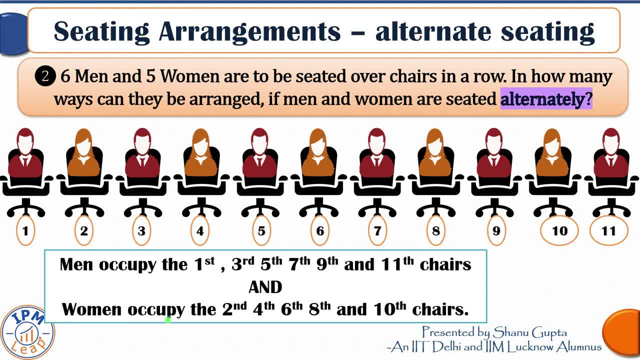 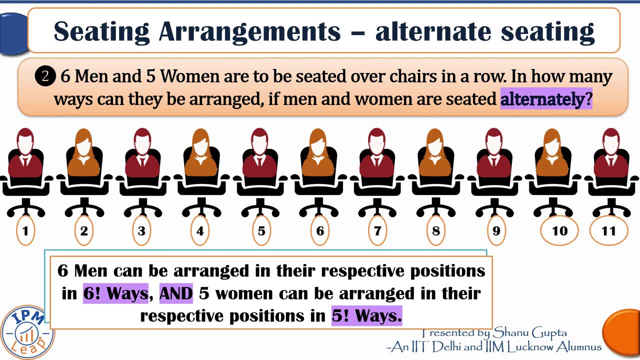 The odd numbered chairs, Women occupy the 2nd, 4th, 6th, 8th and 10th chairs. The even numbered chairs- 6 men- can be arranged in their respective positions in 6 factorial ways And for each of those arrangements, 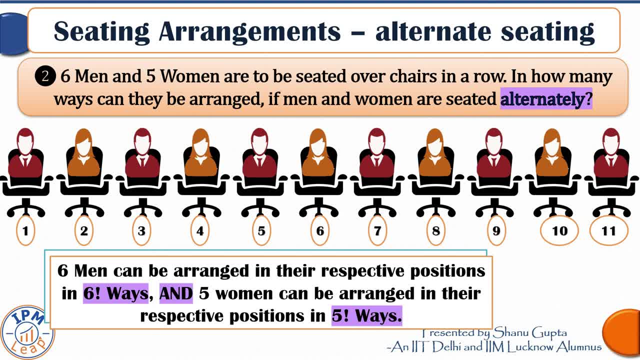 the 5 women can be arranged in their respective positions in 5 factorial ways. Together these men and women can be seated alternately in. Okay, tell me, do we add 6 factorial and 5 factorial or do we multiply 6 factorial and 5 factorial? 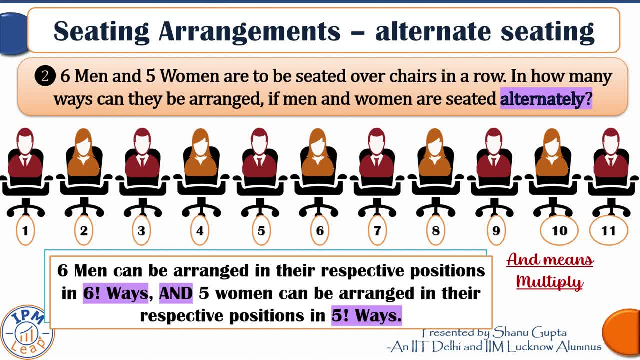 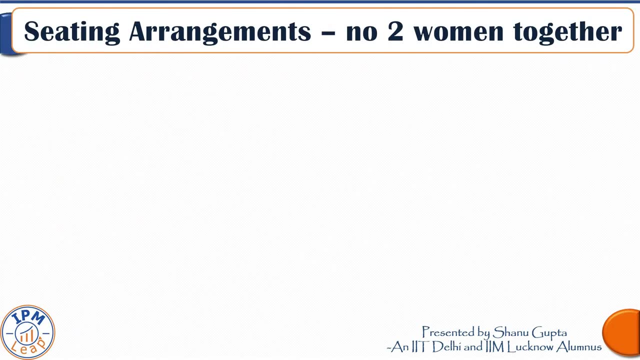 So the answer is because we have to seat men and women and means multiply. So fundamental rule says: multiply the possibilities. Therefore, our answer is 6 factorial into 5 factorial ways for men and women to be seated alternately. Moving on, let us discuss our third constraint. 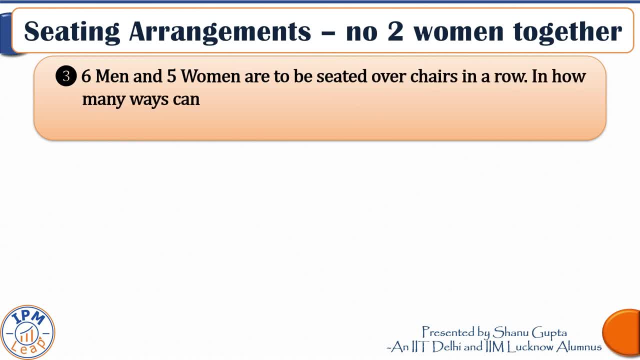 6 men and 5 women are to be seated over chairs in a row. In how many ways can they be arranged if no 2 women are seated together? So, friends, the only difference between this question and the last question of alternate arrangements is that over here, women have to be separated out. 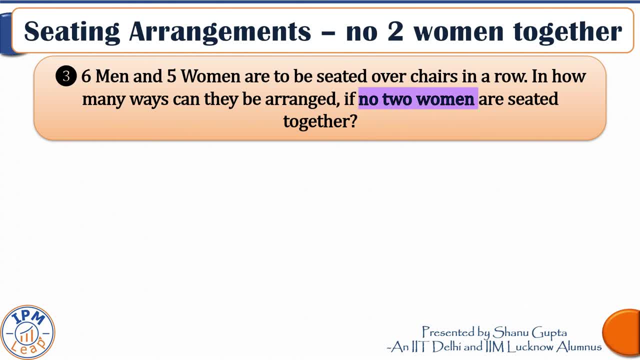 But men could be together. Under the given constraint, 2 or even 3 men could be seated together. It's possible, while the women are all separated out. The way we do such a question is read the phrase no 2: women together. 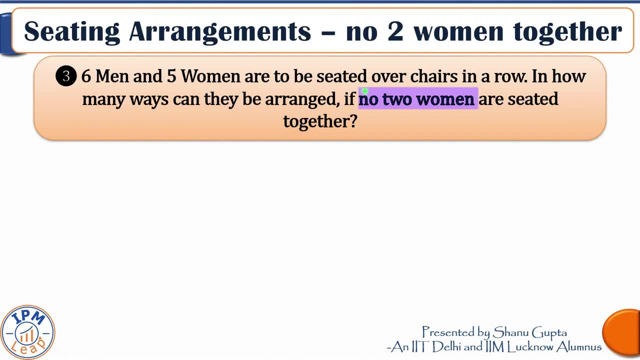 So we need to pick the other category, that is, men, Say, this symbol denotes a man. If we space them out, there will be 5 spaces between the 6 men: 1 space before and 1 space after. So how many spaces? 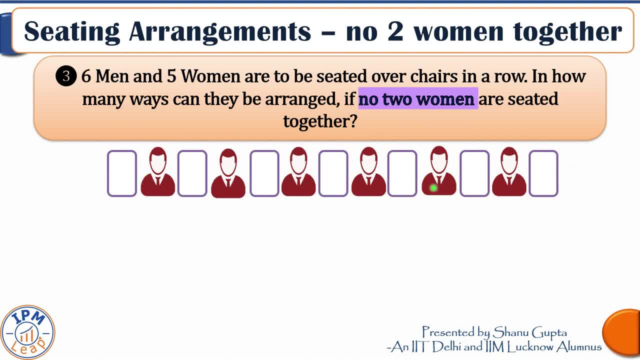 7 spaces in total. These spaces are earmarked for women. We can place maximum 1 woman per space, So 5 women will together occupy any 5 of these spaces out of the given 7.. How many ways of doing that? 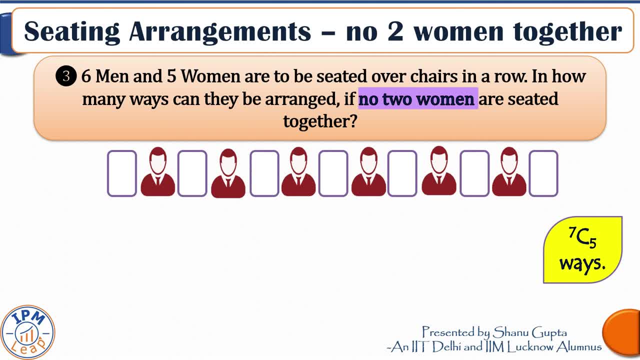 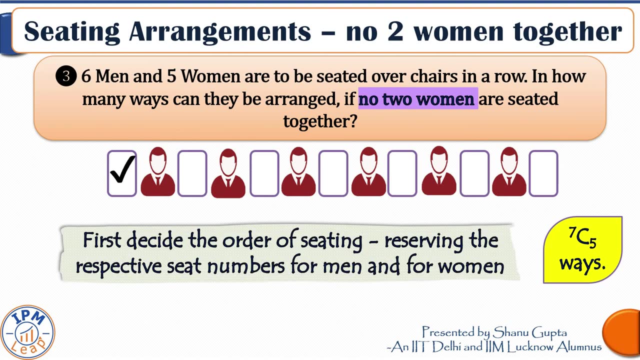 75 ways of doing that. This exercise decides the order of seating. It reserves the respective seat numbers for men and for women. Supposing we selected this space, This one, this one, this one and this one for a female, This would mean the order of seating males and females is already decided. 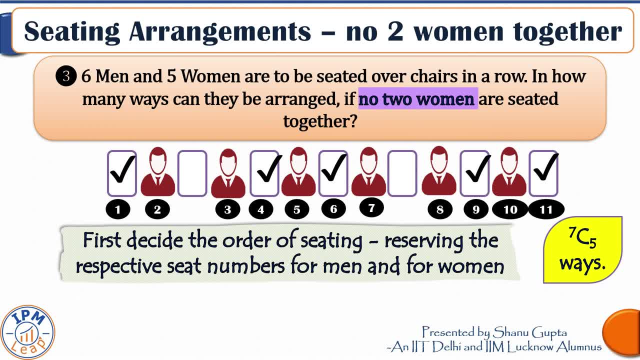 In this case, the 1st, 4th, 6th, 9th and 11th seats or positions are earmarked for a woman And, as the question statement required, no 2 women are together in this. Just make a note here. 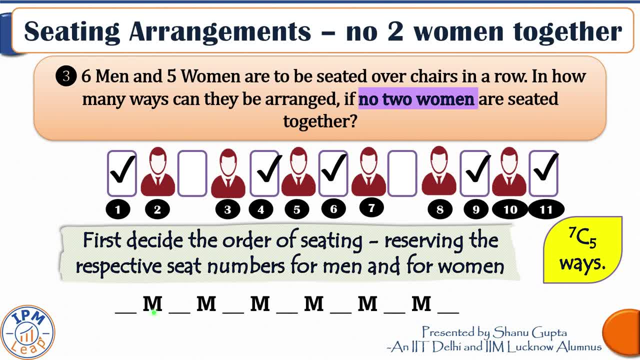 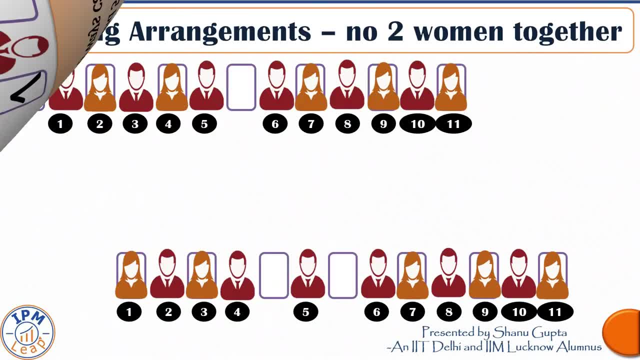 The easier way to do this was to use the letter M for a man instead of the symbol and spaces like these ones. This is another possible arrangement where we see these 2 men on the 5th and 6th seats will be together. 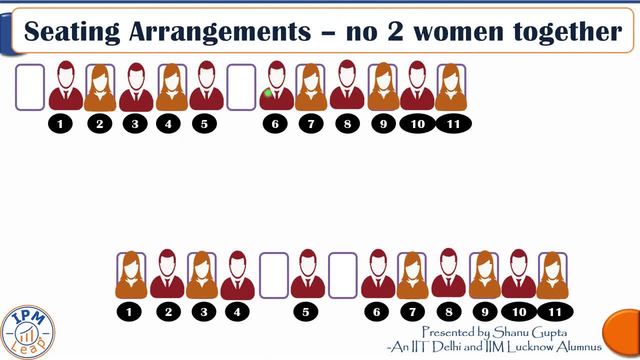 But no 2 women are seated together. still, And this is yet another possible arrangement where we see these 3 men on the 4th, 5th and 6th seats, But, as the question stipulates, no 2 women are seated together in this arrangement as well. 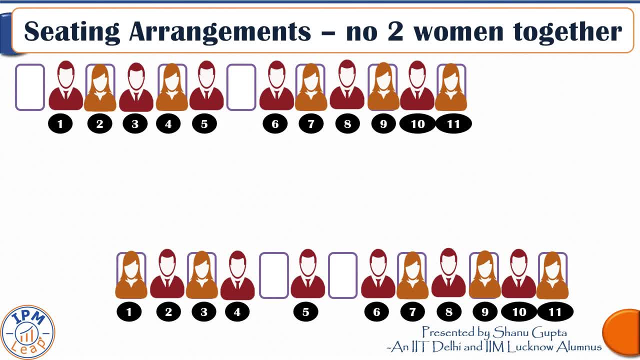 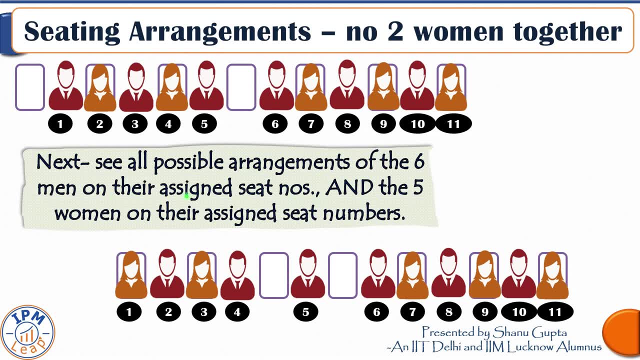 Once we have decided the respective positions of men and women, We can then arrange the 6 men on their assigned seats in 6 factorial ways And the women on their assigned seats in 5 factorial ways. So for our answer, we multiply both steps. 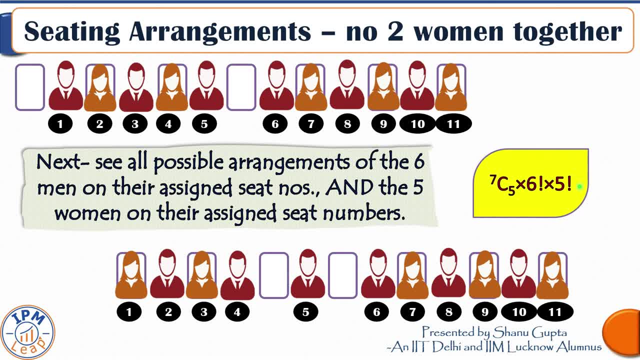 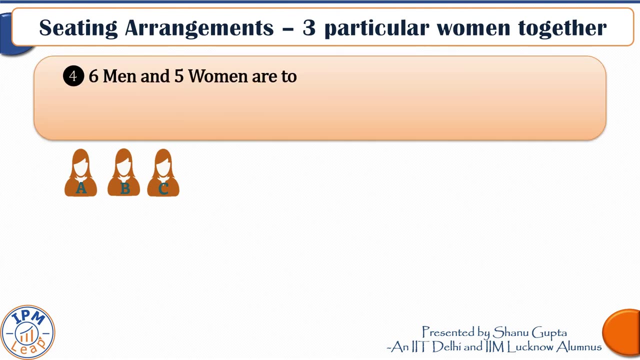 25 x 6 factorial x 5 factorial. That's our answer for no. 2 women seated together And interestingly, in this answer the possibility of alternate arrangements is included. one And finally for our last constraint, wherein we have to seat 3 particular women together. 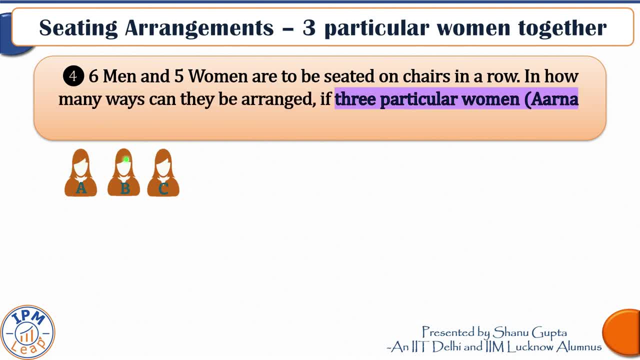 Let's name the 5 women as follows: Aarna, Bhavna, Charu, Driti and Isha- In short, A, B, C, D and E. Now A, B and C need to be seated together.